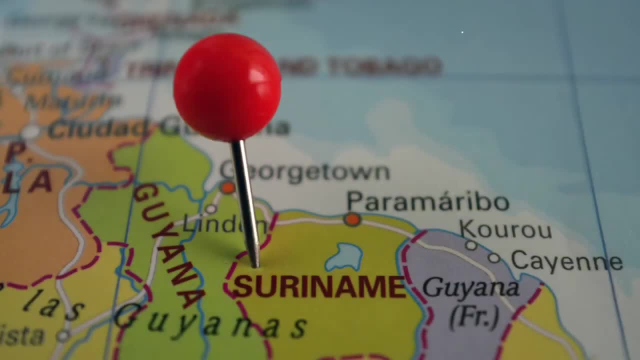 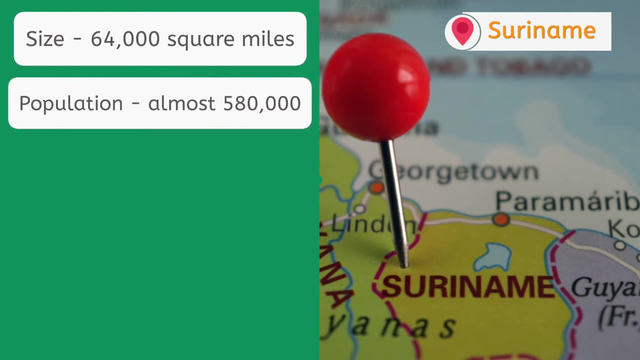 Suriname. Just to the west is Suriname, an independent nation with almost double the size and population of French Guiana. Just over half of Suriname's population is of Asian descent, many of them East Indians or Javanese, while about 30% of the population is French Guiana. 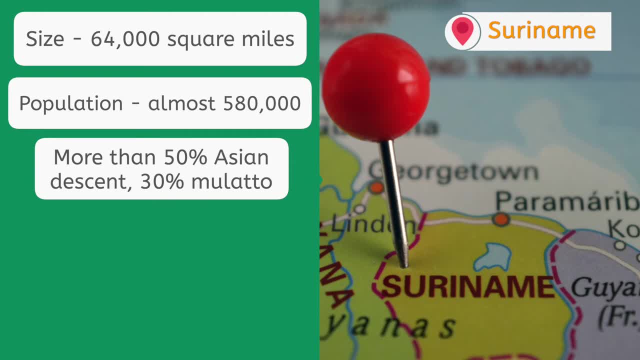 Suriname is classified as mulatto Suriname, a Dutch territory until its 1975 independence and formerly called Dutch Guiana, features a republic form of government. More than half of the population is Christian, but Hinduism and Islam also have a significant number of followers as well. 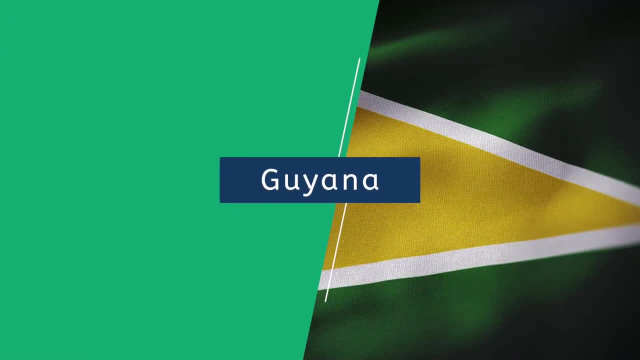 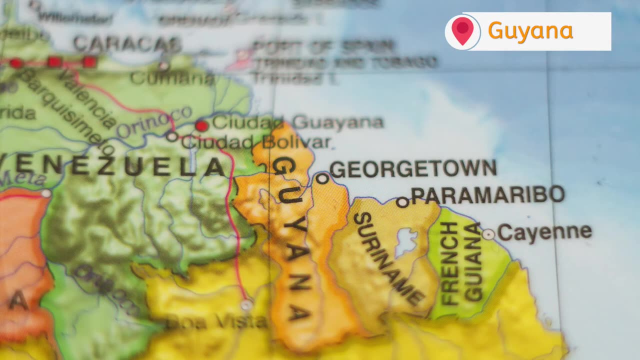 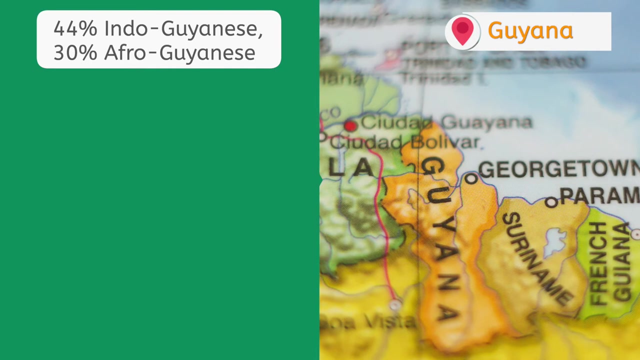 Dutch is the official language Guiana. Like Suriname, Guiana is a republic with a similar but even more diverse blend of religious traditions. Most people in Guiana are of Asian or African descent, and the terms Indo-Guyanese and Afro-Guyanese are used to describe their heritage. 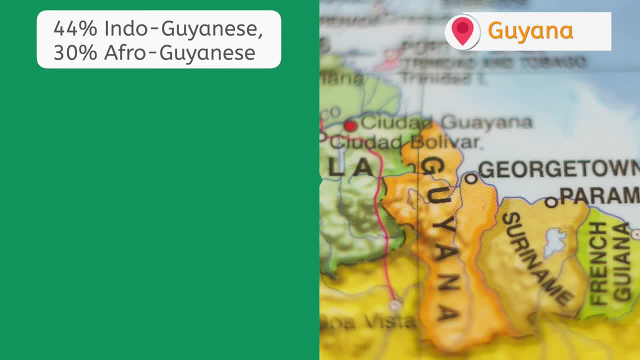 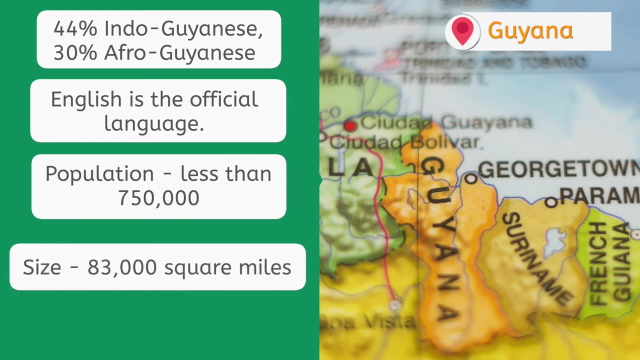 Guiana gained its independence from Great Britain in 1966, but remains part of the British Commonwealth, similar to the Bahamas and Jamaica and the Caribbean. English is the official language for a population of just under 750,000.. At 83,000 square miles, Guiana is similar in size to Utah or 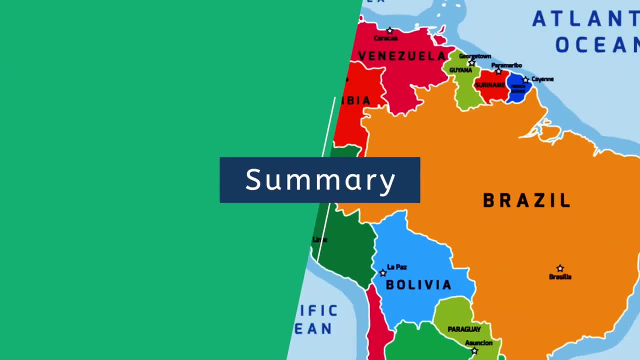 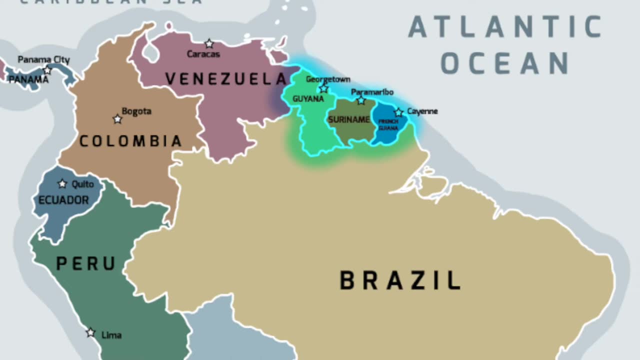 Idaho in the US Summary. The majority of the population of all three- Guiana, Suriname and French Guiana- live in a narrow coastal plain in cities such as Georgetown. Guiana, Paramaribo, Suriname and Cayenne. French Guiana. 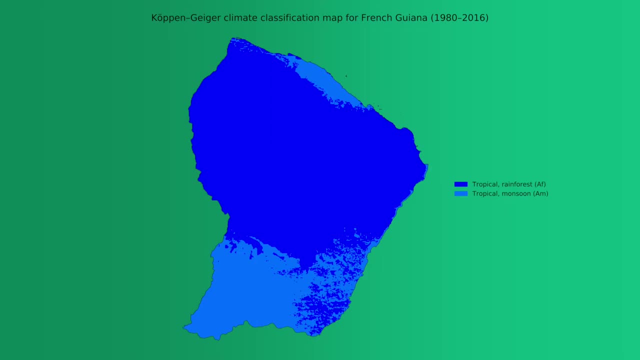 The southern portions of each are dominated by the Amazon Basin and rainforest. The climate of the three ranges mostly from tropical monsoon to tropical rainforest. As an example, check out this climate map of French Guiana. The variety and ethnic composition of these countries reflects the migration patterns of their ancestors. 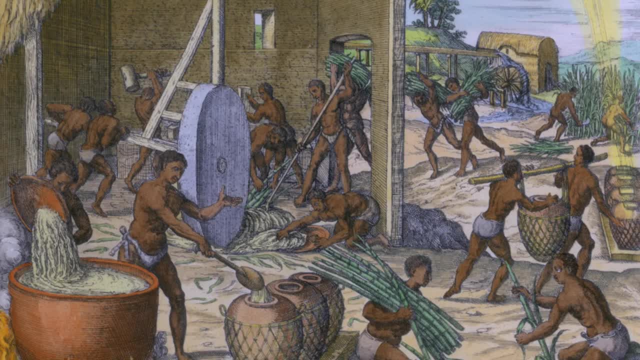 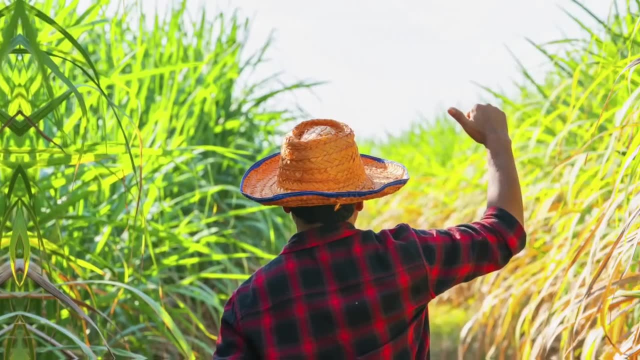 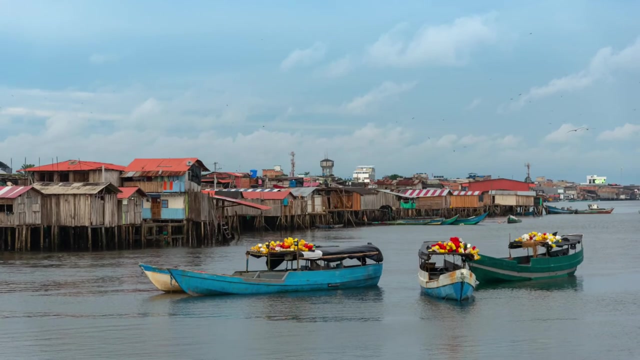 Europeans brought enslaved Africans to labor on sugar plantations. After slavery was abolished, large numbers of Asian workers arrived for those agricultural jobs. Farming remains the basis of the economy in all three nations, as sugarcane and rice are major crops. The primary economic activity of fishing also provides work for farmers. 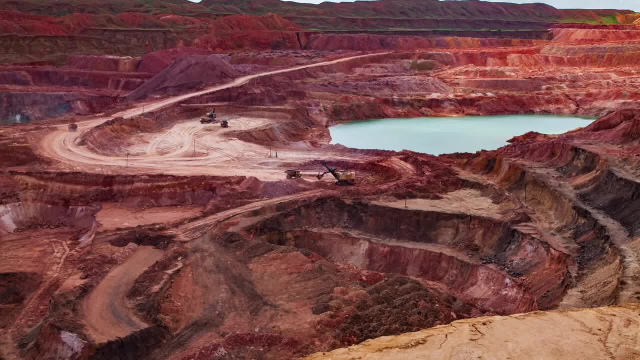 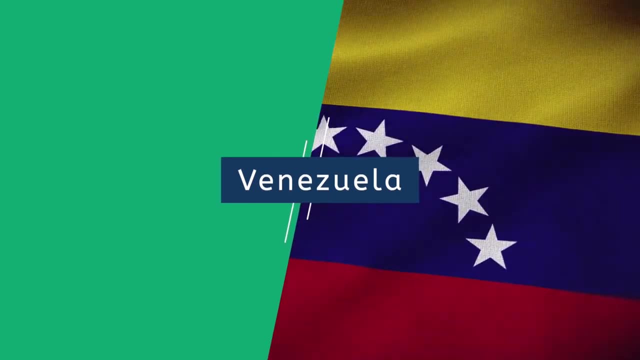 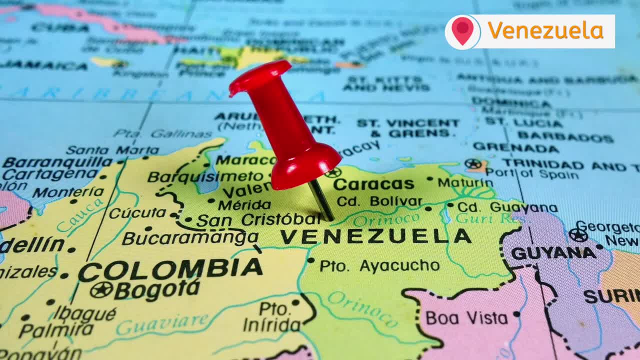 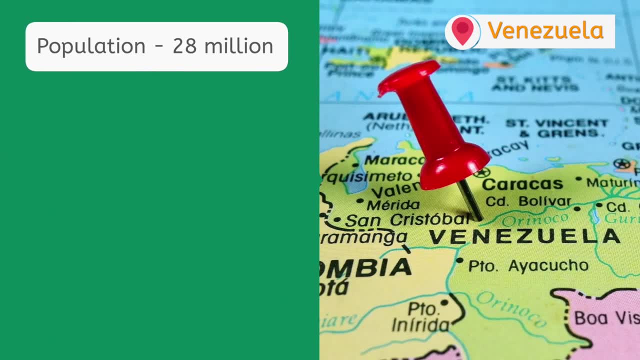 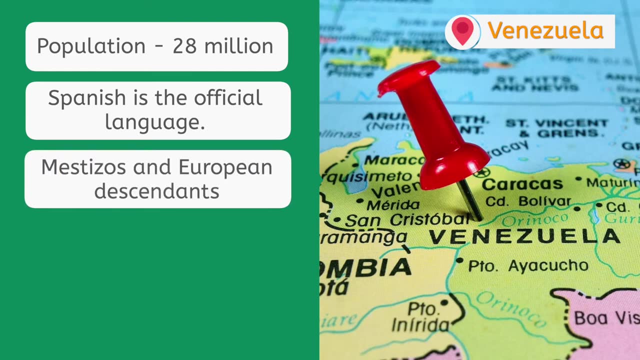 the Antemunic waking up to the sea allows united nations to wonder and study and use the oceans out into their own and along bottom, White Cretaceous, White Cretaceous, Household Miners, Household Miners, Household Miners. Number eight GROUP, those of European descent. Largely because of that heritage, 71% of Venezuela's residents are 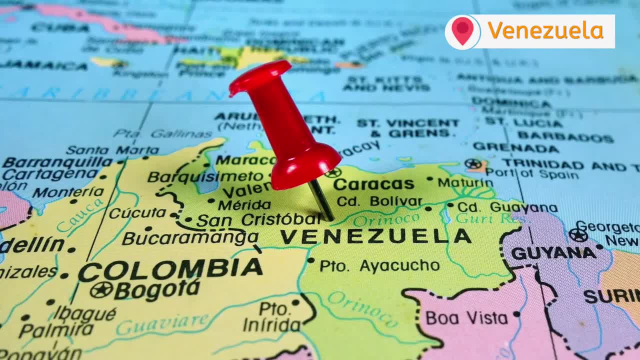 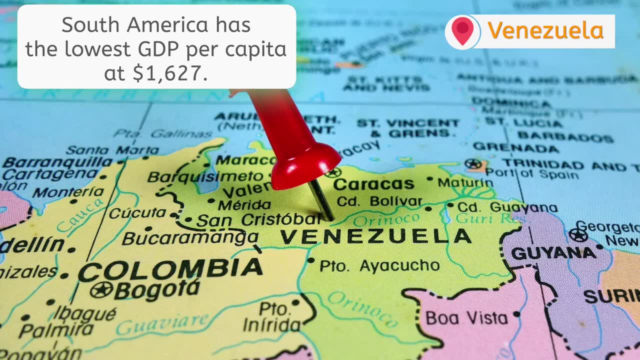 Roman Catholic. Despite a mixed economy based on petroleum production, Venezuela has the lowest GDP per capita in South America, at just over US$1,600 as of 2021.. This despite Venezuela's status as one of the world's top exporters of petroleum and owner of the world's largest oil. 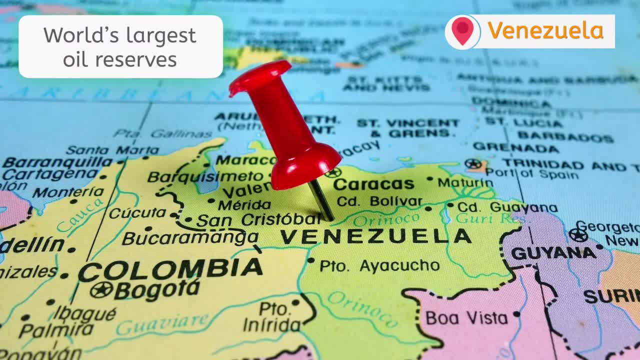 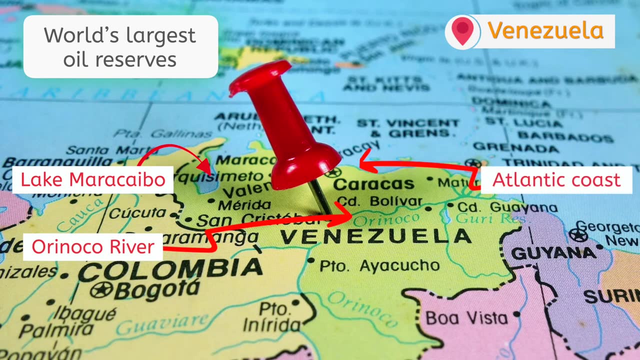 reserves. You heard that right. Venezuela has the world's largest oil reserves. Those are spread out among three primary locations around and beneath Lake Maracaibo in the northwest part of the country, the Orinoco River and Delta in the east, and offshore in the Atlantic Ocean. 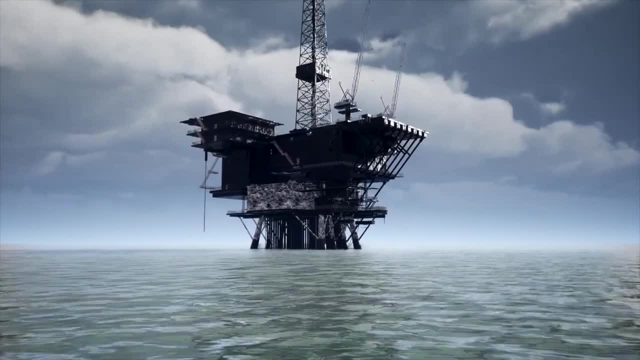 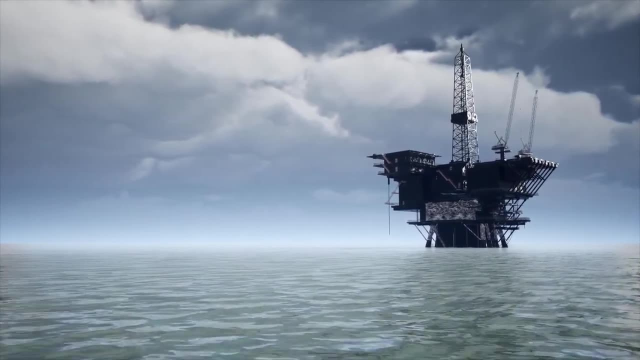 The national revenue of Venezuela is almost completely dependent on oil production, but questionable government policies and decisions have led to a complete collapse of the national economy in 2013.. The result has been a nation troubled with hyperinflation, which is a period of extremely 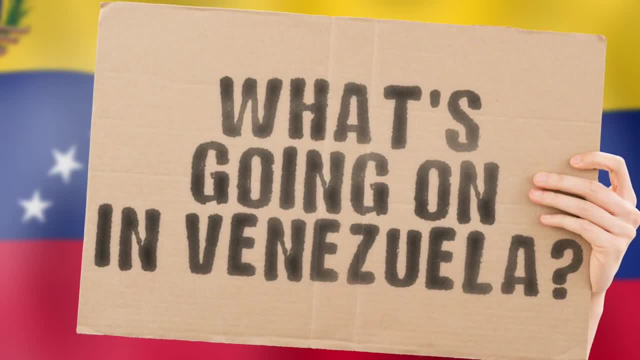 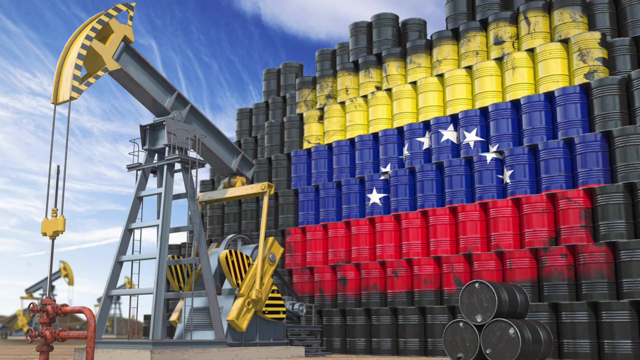 high monetary inflation. Other problems include unemployment, poverty, crime and corruption, attempted mass migrations to the neighboring country of Colombia and shortages of basic goods for its people. Little stimulation for the economy exists other than reliance on petroleum. Much of the agriculture is subsistence farming, but the primary cash crop is coffee. 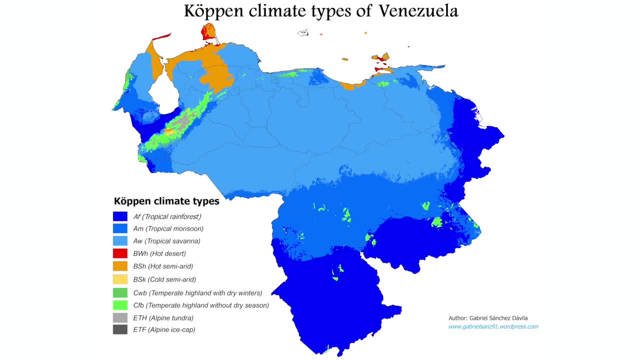 which is harvested and the most important thing is that it is produced in the wild, temperate highlands, shown here in bright green. Overall, the climate for most of Venezuela is predictably tropical, as you can see, with the varying shades of blue that represent the monsoon, rainforest and savanna ranges within the tropical. 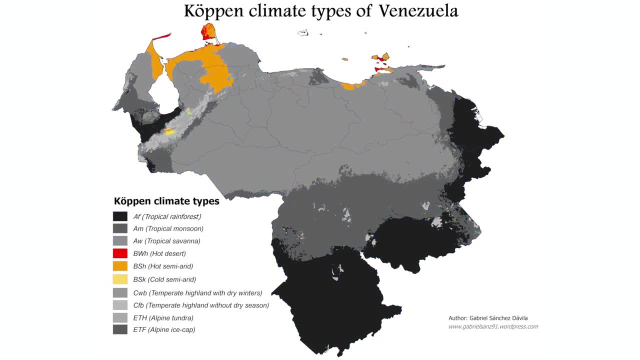 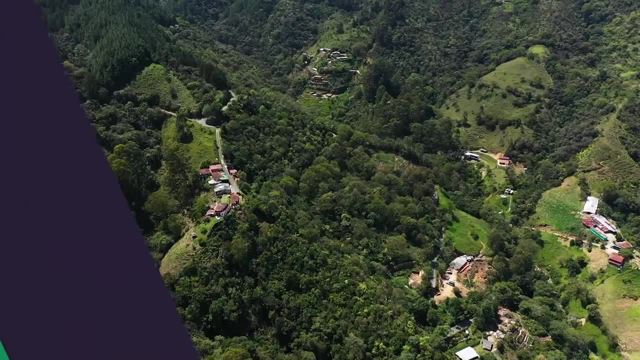 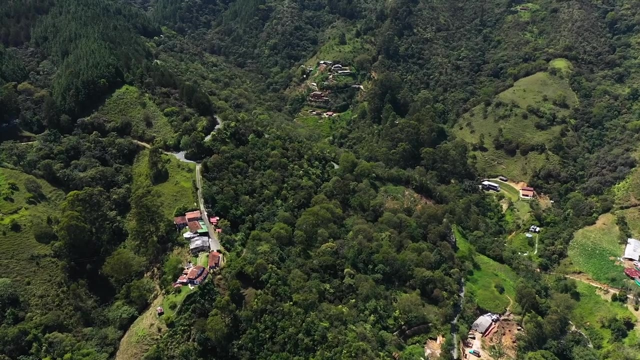 climate Along and near the coast. the orange and red colors of the map reflect small areas with hot, semi-arid and hot desert climate conditions. The landforms of Venezuela are diverse and two physical features dominate the landforms. The first are the Andean highlands, a range of mountains, plateaus and hills stretching over most of northern Venezuela. The capital and largest city, Caracas, is located at the foothills of these highlands along the Atlantic Coast. Most Venezuelans, about 93% in fact, live in these mountain valleys in the northern part of the country. The other most notable physical 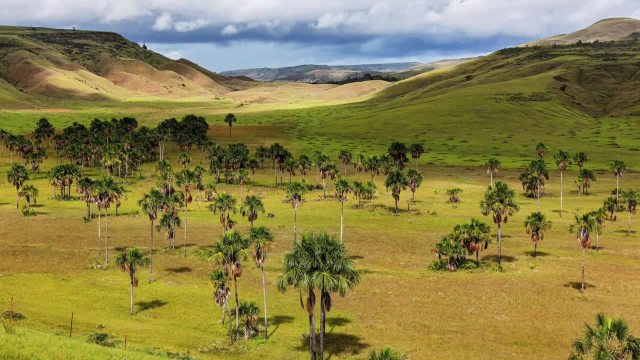 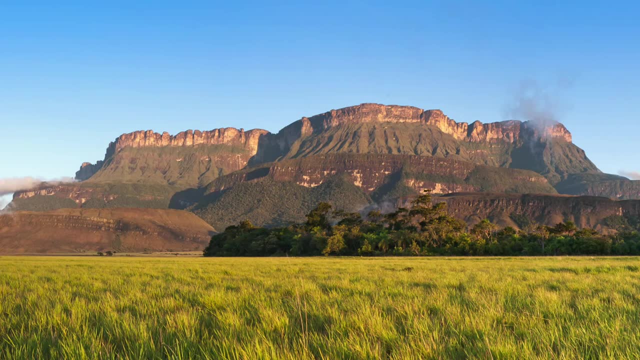 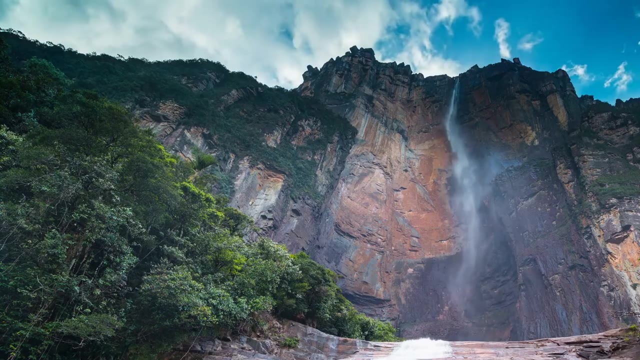 feature of Venezuela is the waterfalls and grasslands of the southeast, While the The Guyana Highlands cover almost half the country. The population there is sparse, but the natural beauty isn't. Angel Falls is located here Now. you've heard of it and probably already know that it's the world's highest waterfall. 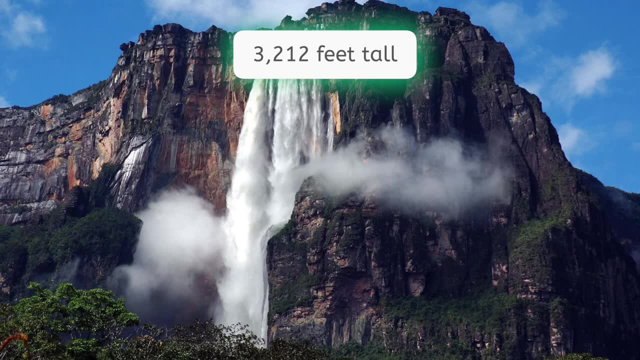 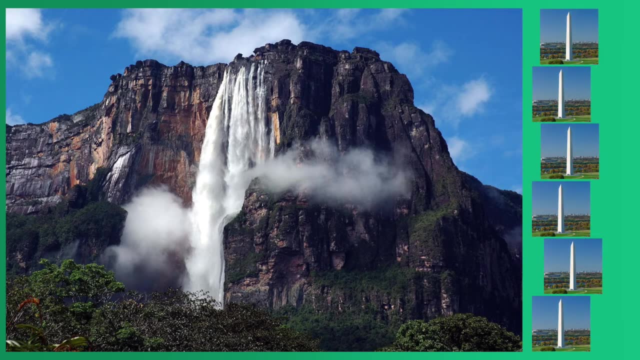 You may not know that its height, 3,212 feet, measures more than half a mile and is nearly six times as tall as the Washington Monument. Venezuela's most important river, the Orinoco, flows through the highland region before emptying. 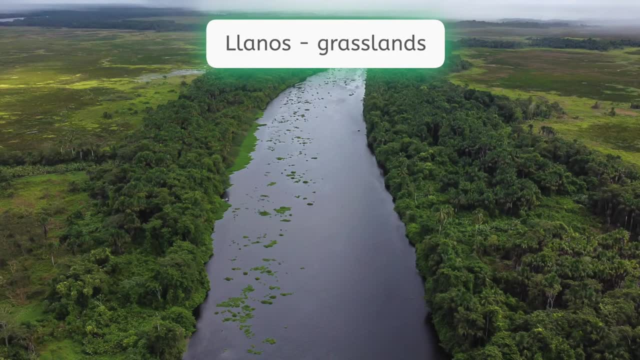 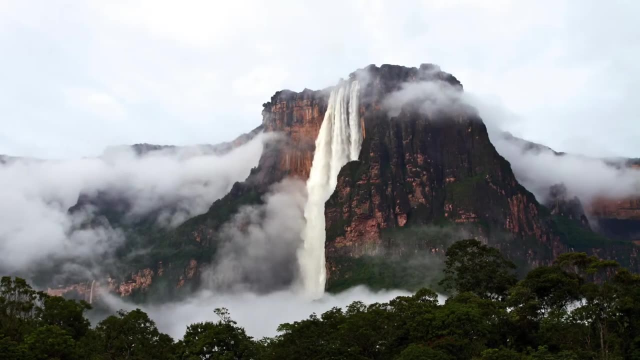 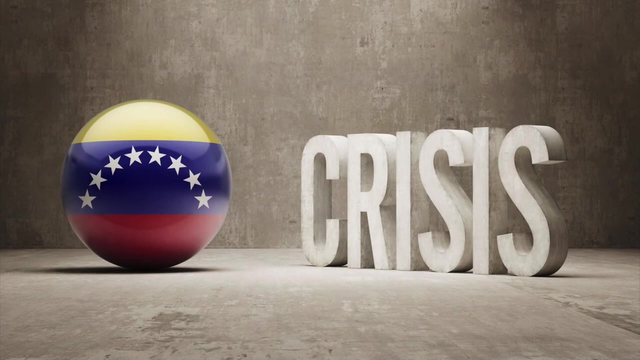 into the Atlantic Ocean. Wide tropical grasslands, called llanos, flank each side of the Orinoco. Despite the ecological diversity and natural beauty, Venezuela, as mentioned earlier, continues to deal with many political and economic issues. Millions fled the country following the 2013 presidential election, due largely to the 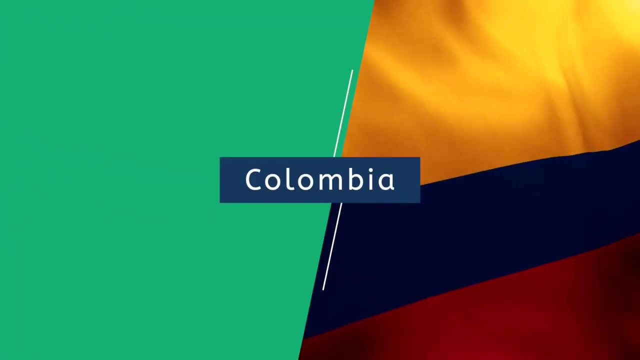 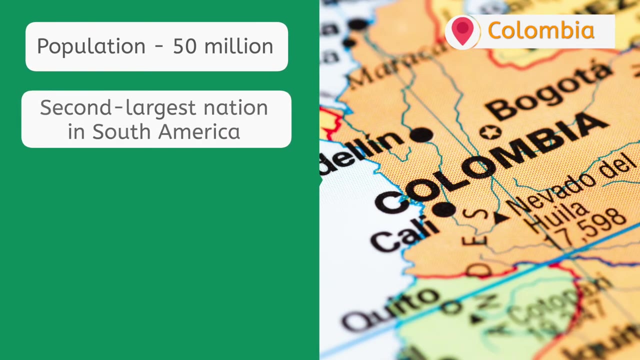 government's instability. Colombia. The second most populous nation in South America is Colombia, whose 50 million citizens trails only Brazil in number. Almost 88% of Colombians did not identify with any ethnic group in the 2018 census and are considered either mestizo or white and of European descent. 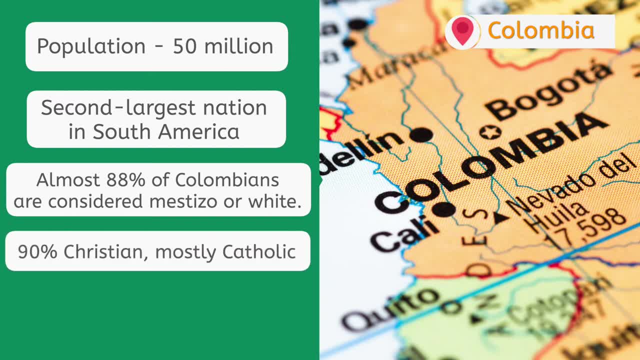 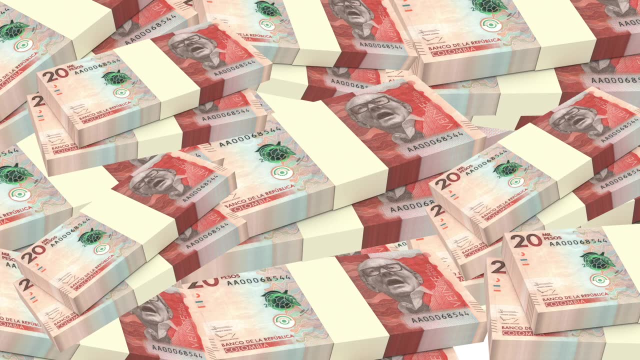 About 90% of Colombians are Christian. The vast majority of those identify as Roman Catholic. Spanish is the official language, but English and Portuguese are recognized as well. Colombia In several Latin American nations. Colombia faces political and economic turmoil from social inequality. 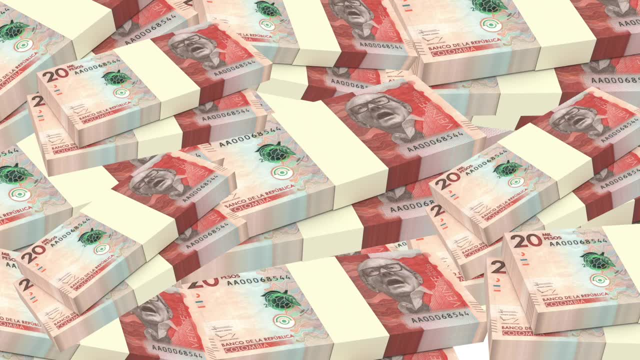 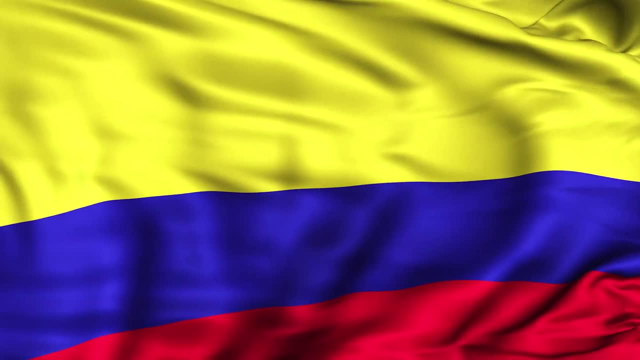 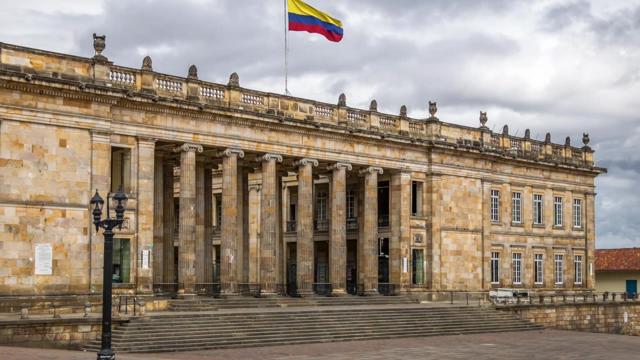 A small percentage of people hold the majority of the nation's wealth and power, while many suffer extreme poverty. Such disputes and civil strife linger despite a civil war between the two main political parties in the 1950s. Foreign policy in Colombia has delegitimized the government in the past as money flowing. 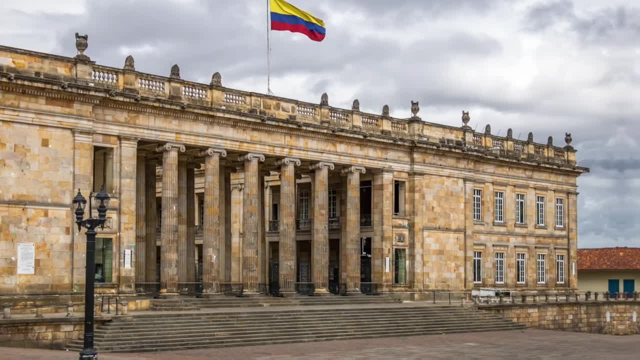 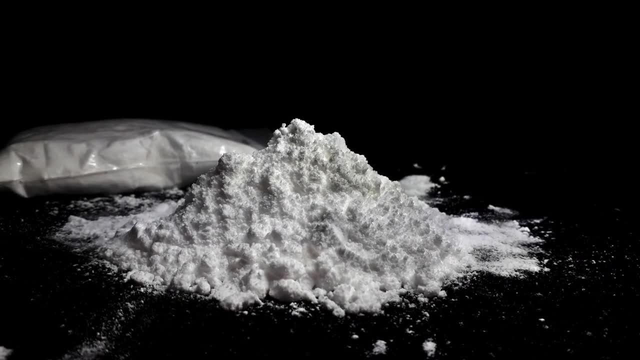 into the nation was intended to wipe out the drug trade. Colombia's drug trade has been a major threat to the country. Instead, much of Colombia remains involved in the production and sales of marijuana and cocaine, among others, which bring huge profits to the drug cartels and, in many cases, provide 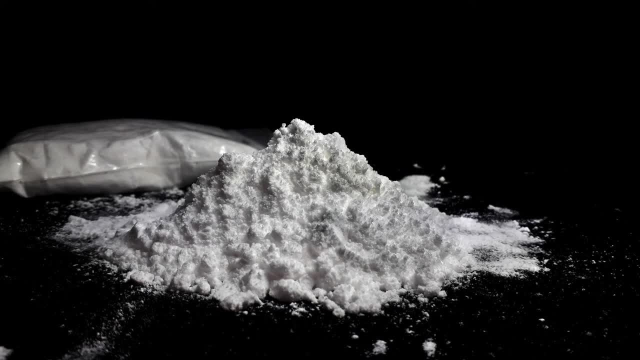 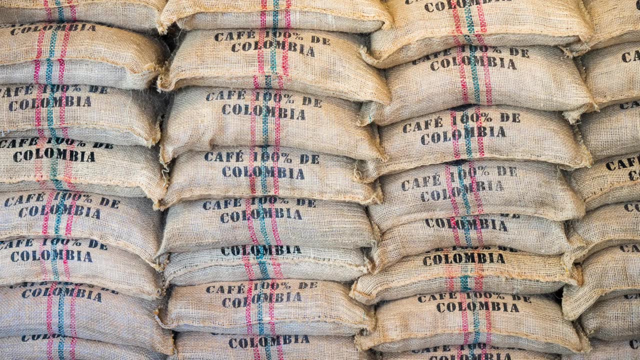 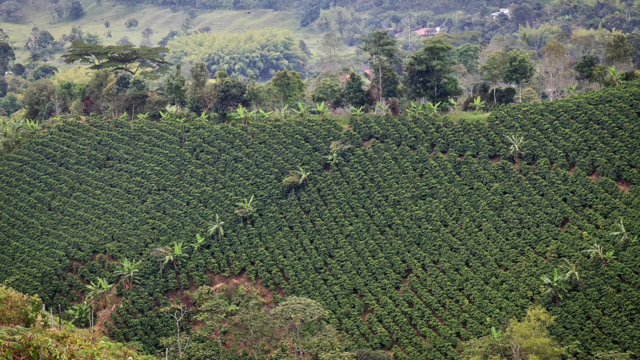 more financial reward for Colombians than other types of crops. The Colombian economy is highly dependent on coffee for legal revenue, so much so that the nation is at times considered monoculture, which is the cultivation of a single crop in a given area. Coffee beans are grown on hundreds of thousands of acres of land. 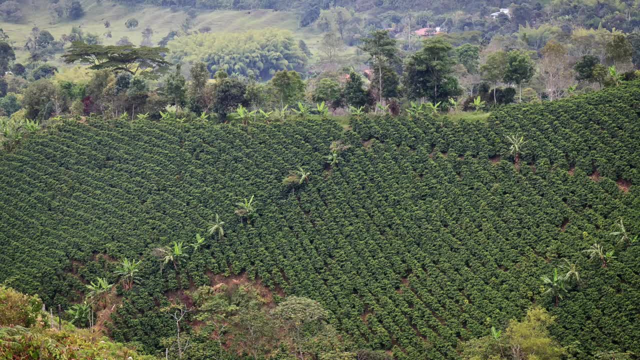 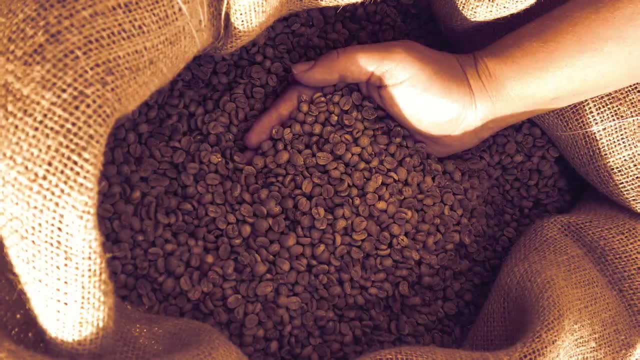 There are hundreds of thousands of small farms in Colombia, But most farmland is owned by a handful of wealthy families who rent at high prices to tenant farmers called campesinos, a system very similar to sharecroppers of the American South following the US Civil War. 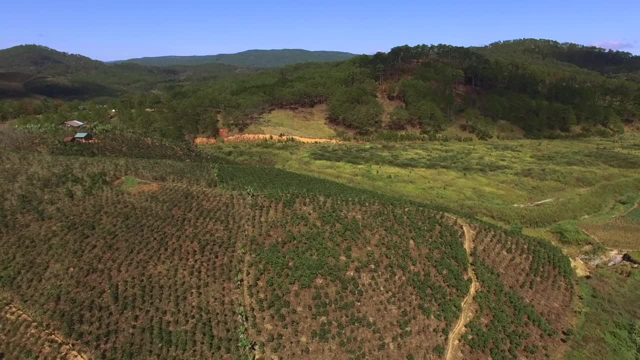 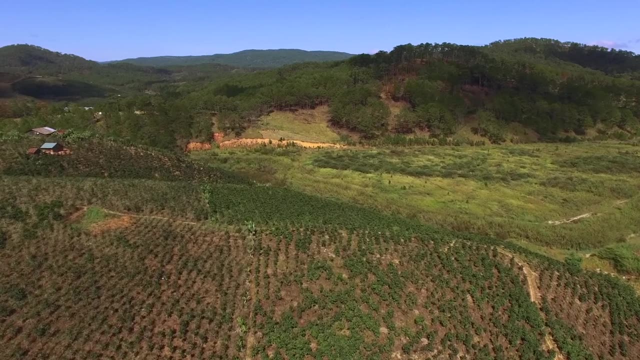 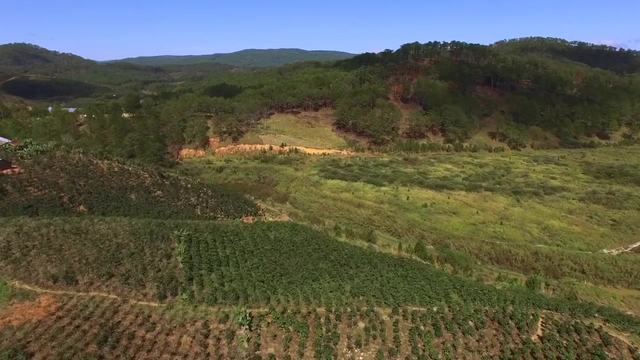 The physical characteristics and climate of Colombia make it near perfect for growing coffee. The landscape is dominated by the Andes Mountains, the lowlands and the llanos, as the vast majority of its 50 million inhabitants are Colombian. million citizens live in the fertile valleys between three cordilleras or mountain ranges. 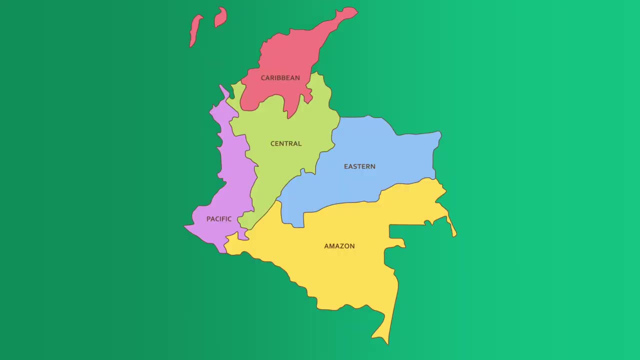 of the Andes. The climate, while often characterized as tropical, actually offers considerable variation based on the natural regions found within Colombia. Those regions are based on altitude, temperature, humidity, winds and rainfall. Climate zones include tropical, rainforest, savanna, steppe, desert and alpine climate, each dependent on the factors 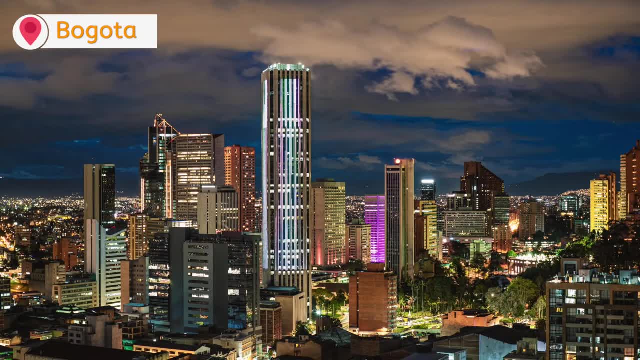 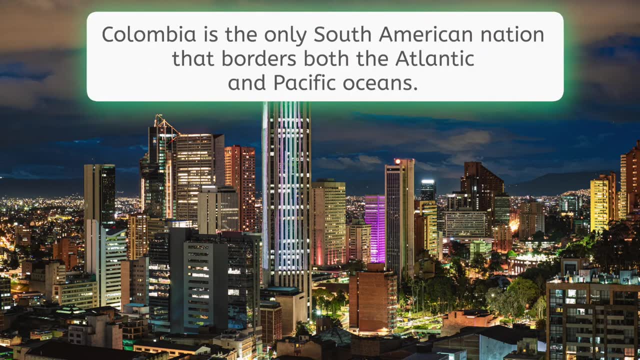 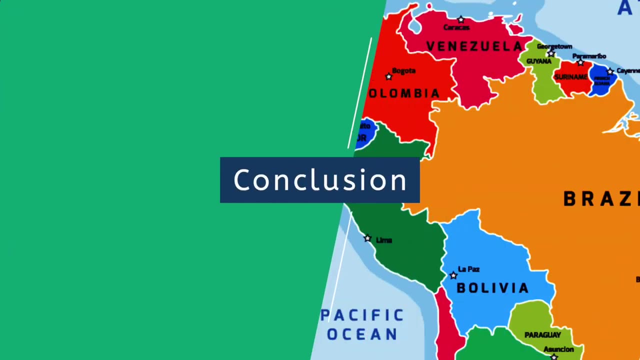 mentioned before, Colombia's largest city and capital is Bogota, located in the heart of the country. One more thing: Colombia is the only South American nation that borders both the Atlantic Ocean's Caribbean Sea and the Pacific Ocean. Conclusion: The geography of South America's. 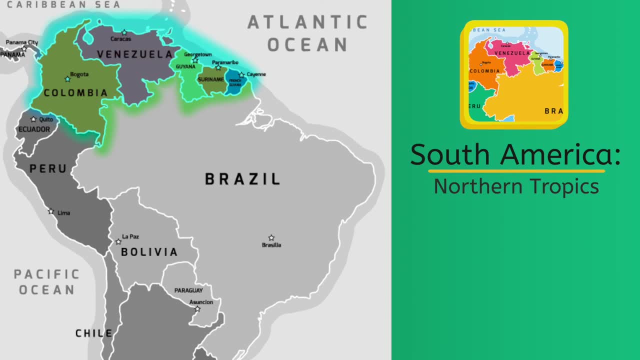 northern tropics region is varied but defined. It is defined largely by the topography of the Andes Mountains, the Amazon Rainforest and the Atlantic Coast. Cultural groups and nations are split by these physical features and past migrations, creating vibrant and varied nations facing economic and governmental. 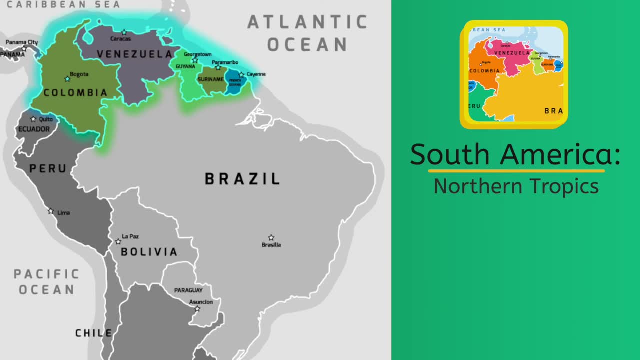 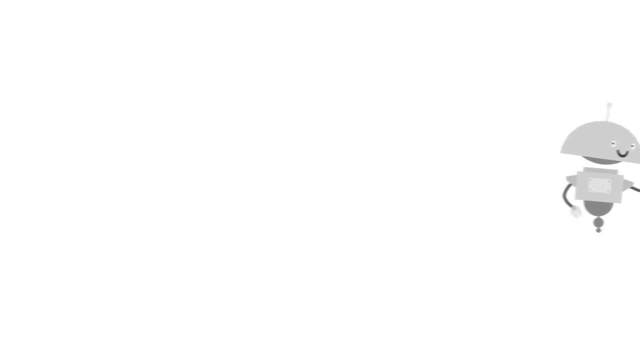 challenges. Until next time, keep exploring. Transcription by CastingWords.